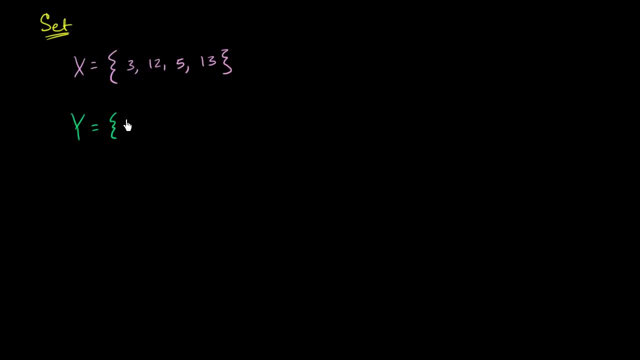 it's a set. It's a set. It's a collection of the distinct objects: the number 14,, the number 15,, the number 6, and the number 3.. So, fair enough, Those are just two set definitions. 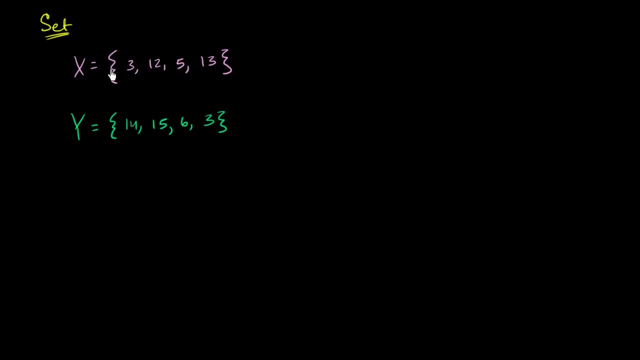 The way that we typically do it in mathematics is we put these little curly brackets around the objects that are separated by commas. Now let's do some basic operations on sets, And the first operation that I will do is called intersection. So we would say x intersect, the intersection of x and y. 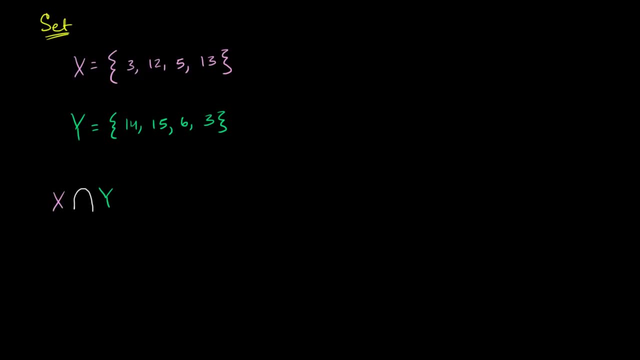 And the way that I think about this, this is going to yield another set that contains the elements that are in both x and y, So I often view this intersection symbol right here as and So all of the things, things that are in x and in y. 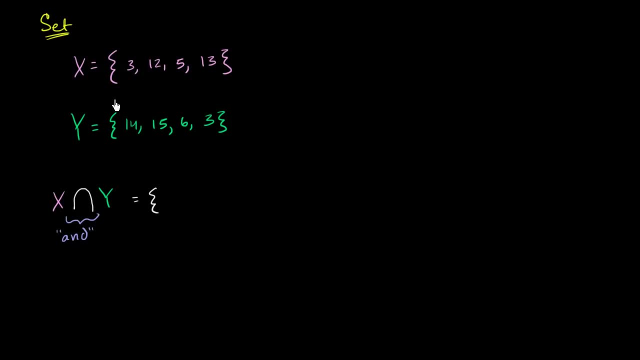 So what are those things going to be? Well, let's look at both sets x and y. So the number 3 is in set x. Is it in set y as well? Well, sure, It's in both, It's in both. so it will be in the intersection of x and y. 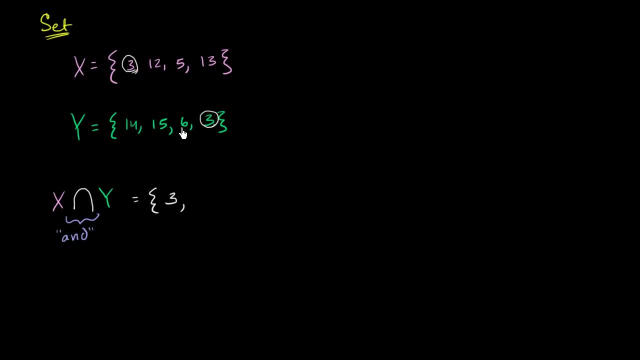 Now the number 12, that's in set x but it isn't at y, So we're not going to include that. The number 5, it's in x but it's not in y. And then we have the number 13: is in x but it's not in y. 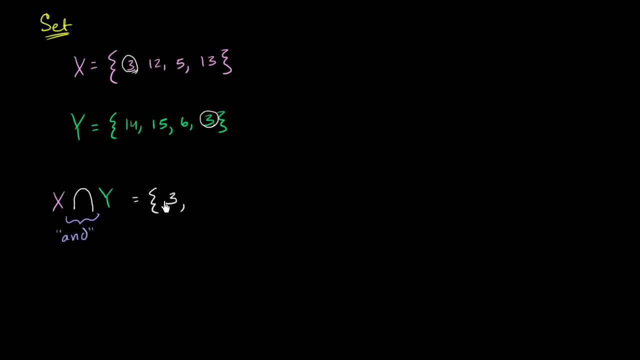 And so over. here the intersection of x and y is the set that only has one object in it. It only has the number 3.. So we are done. The intersection of x and y is 3.. Now another common operation on sets is union. 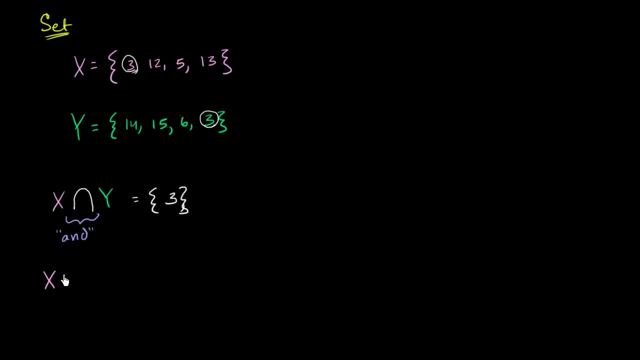 So you could have the union, The union of x, x and y And the union I often view, or people often view as or. So we're thinking about all of the elements that are in x or y. So in some ways you can kind of imagine. 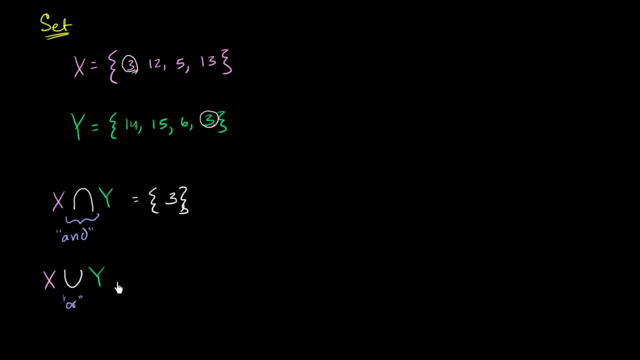 that we're bringing these two sets together. So this is going to be- and the key here is that a set is a collection of distinct objects And the way we're conceptualizing things right here. this is the number 3.. This isn't like somebody's score on a test. 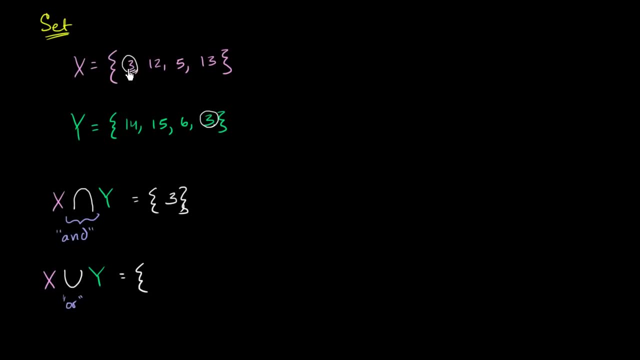 or the number of apples they have, And so there you could have multiple people with the same number of apples. Here we're talking about the object, the number 3. So we can only have a 3 once. But a 3 is in set, is in x or y. 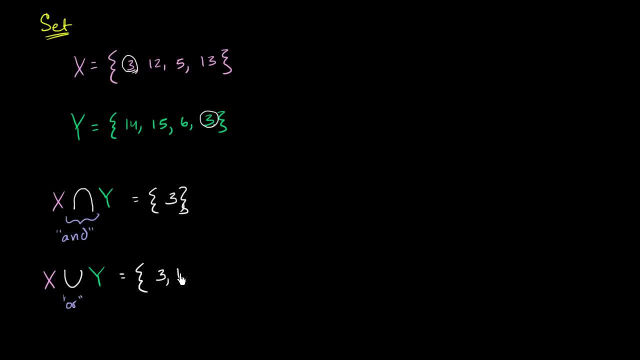 So I'll put a 3 there, A 12 is in x or y, A 5 is in x or y, The 13 is in x or y, And just to simplify things, we really don't care about order if we're just talking about a set. 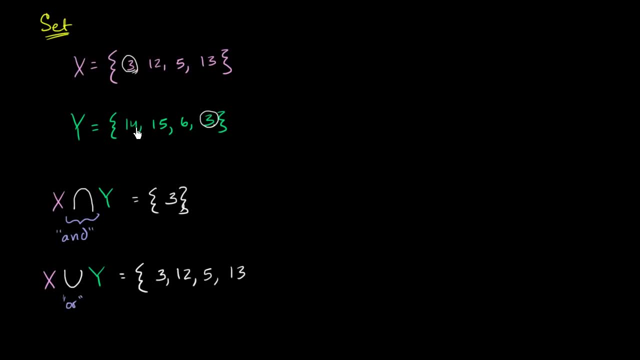 I've just put all of the things that are in set x here, And now let's see what we have to add from set y. So we haven't put a 14 yet. So let's put a 14.. We haven't put a 15 yet. 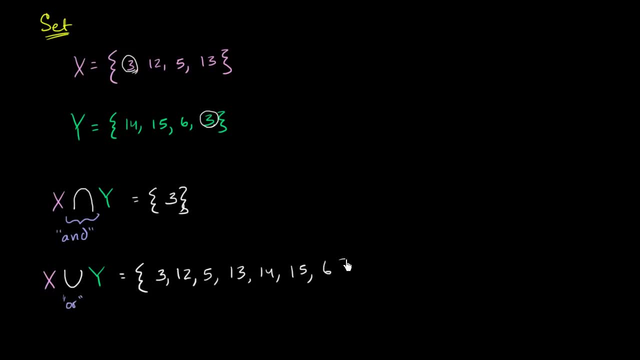 We haven't put the 6 yet And we already have a 3 in our set. So there you go. You have the union of x and y, And one way to visualize sets and visualize intersections and unions and more complicated things is using a Venn diagram. 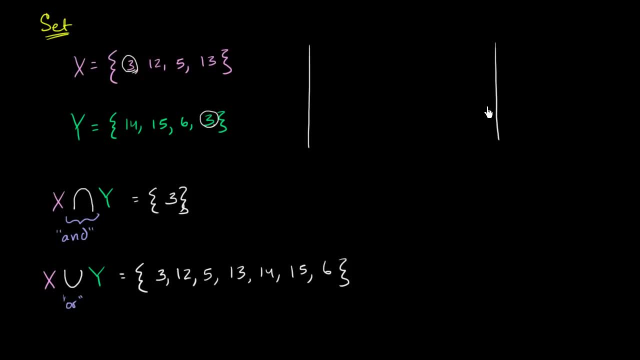 So let's say, this whole box is- you could do that- it's a set All numbers. So that's all the numbers right over there. We have set x. I'll just draw as a circle right over here And I could even draw the elements of set x. 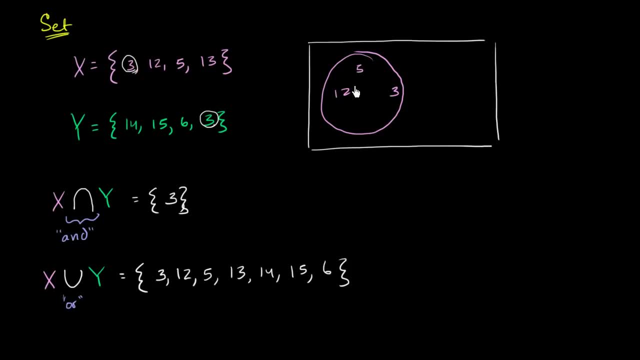 So you have 3 and 5 and 12.. 3,, 5,, 12, and 13.. And then we can draw, set y And notice I drew a little overlapping here because they overlap at 3.. 3 is an element. 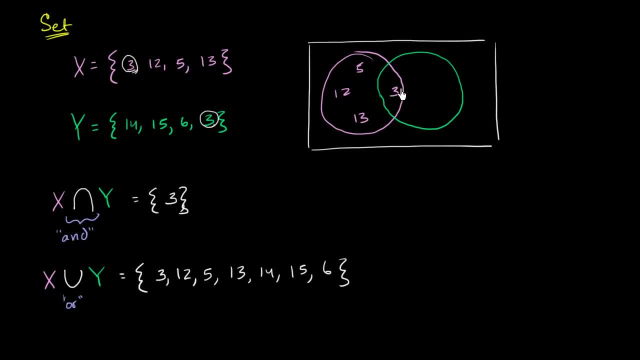 In both set x and set y. But set y also has the numbers 14,, 15, and 6.. And so when we're talking about x intersect y, we're talking about where the two sets overlap. So we're talking about this region right over here. 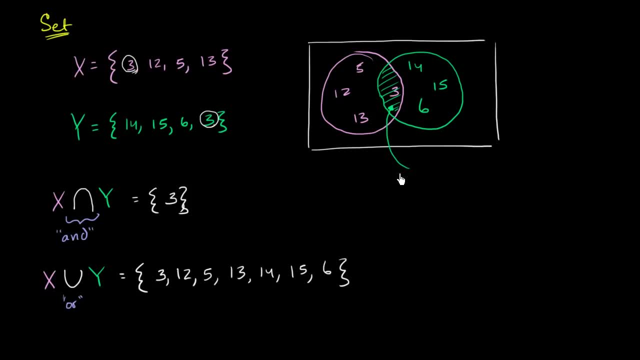 And the only place that they overlap the way I've drawn it is at the number 3.. So this is x intersect y, And then x union y is the combination of these two sets. So x union y is literally everything, everything right here that we are combining. 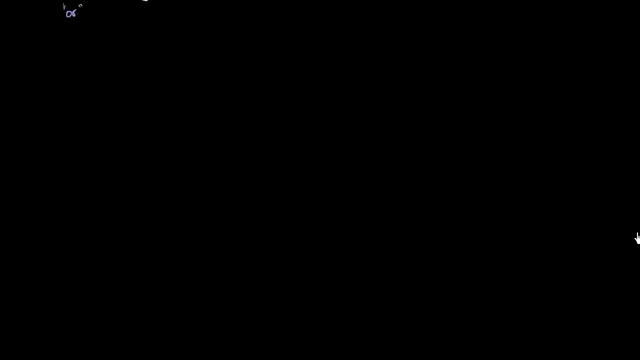 Let's do one more example just so that we make sure we understand intersection and union. So let's say that I have set a, And set a has the numbers 11,, 4,, 12, and 7 in it, And I have set b. 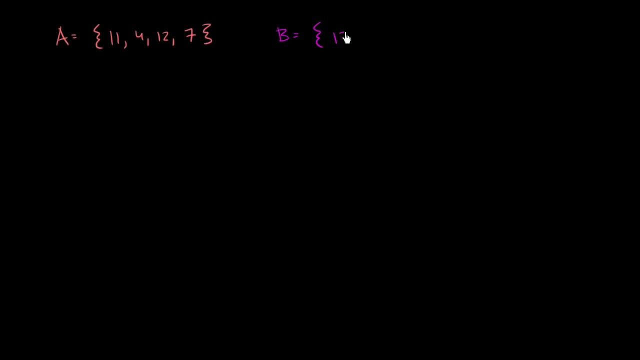 I have set b And it has the numbers 13,, 15, and 6.. 4,, 12,, 10, and 3 in it. So first of all, let's think about what a. Let me do that in a's color. 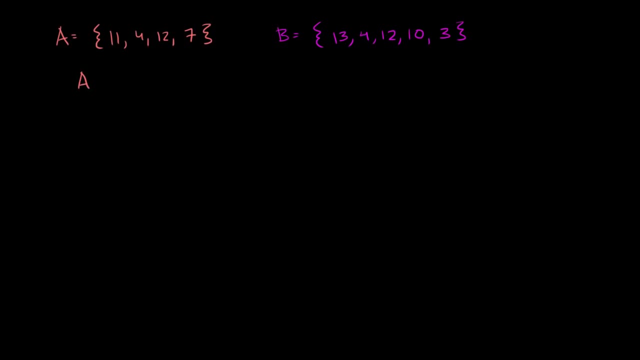 Let's think about what a intersect b is going to be equal to. Well, it's the things that are in both sets. So I have 11 here. I don't have an 11 there, So that doesn't make the intersection. 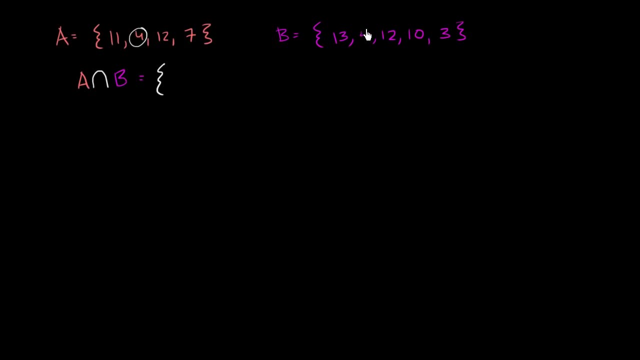 OK, So that doesn't make the intersection. I have a 4 here, I also have a 4 here. So 4 is in a and b. It's in a and b, So I'll put a 4 here, The number 12, it's in a and b. 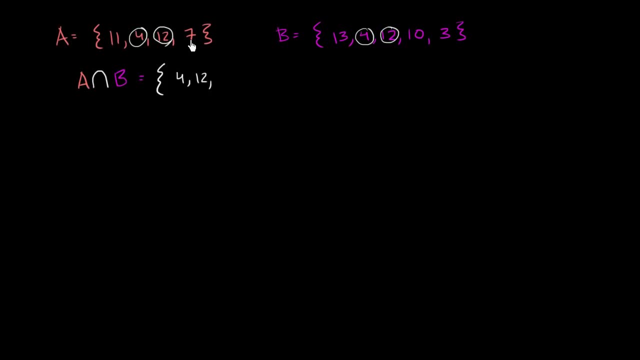 So I'll put a 12 here. Number 7 is only in a And then number I guess 13,, 10, and 3 is only in b. So we're done 4 and 12,. the set of 4 and 12 is the intersection of sets a. 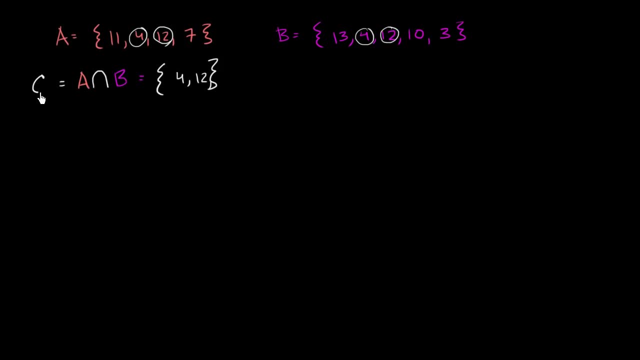 and b, And we could even, if we want to, we could even label this as a new set. We could say set c is the intersection of a and b And it's this set right over here. Now let's think about union. 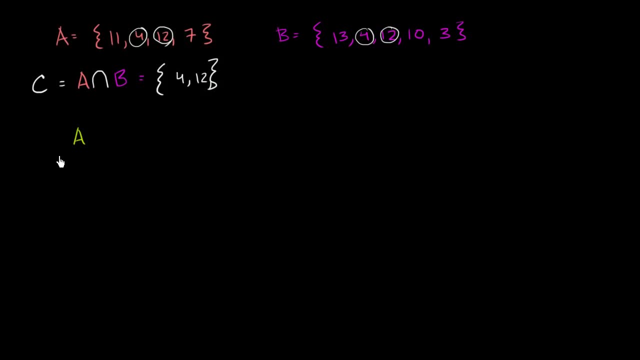 Let's think about a. I want to do that in orange. Let's think about a union, a union, b. What are all the elements that are in a or b? Well, we can just literally put all the elements in a: 11,, 4,, 12,, 7..